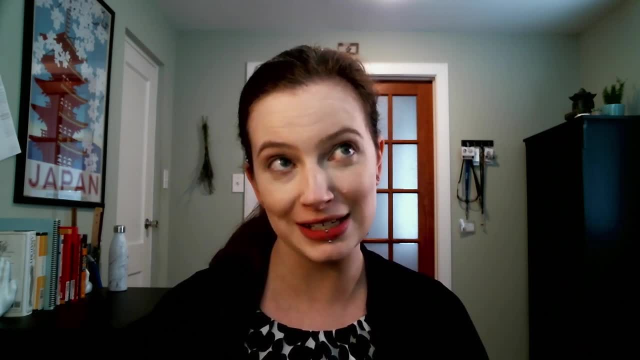 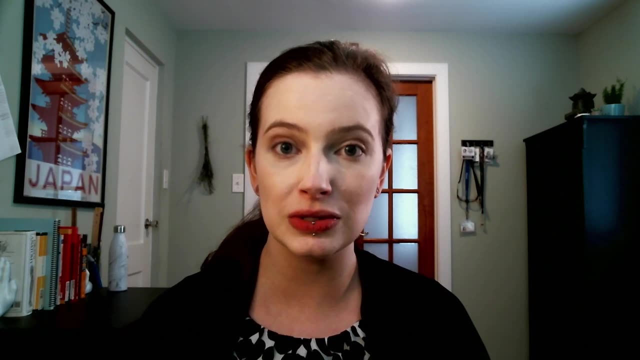 time, Even if we include in our pre-session. please speak in short phrases. oftentimes people aren't going to speak in short phrases, no matter how many times we remind them, So we need to use our consecutive practice as an opportunity to improve our memory retention. Tip number three: 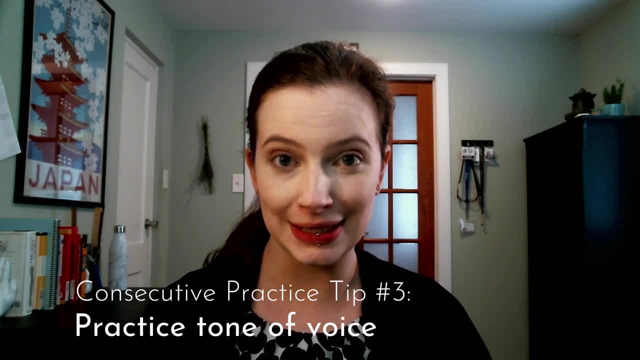 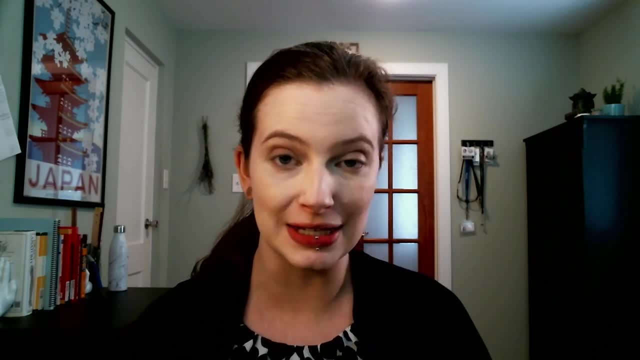 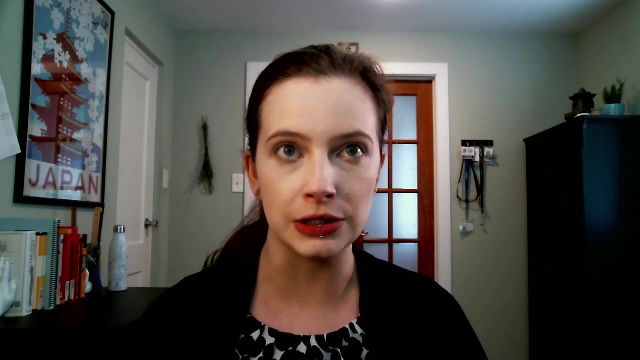 is practice, tone and intonation, as well as inflection. when you are interpreting, When you're practicing with consecutive. let's face it: when a patient is speaking or when a provider is speaking in the field, they're not going to speak in monotone, So you shouldn't. 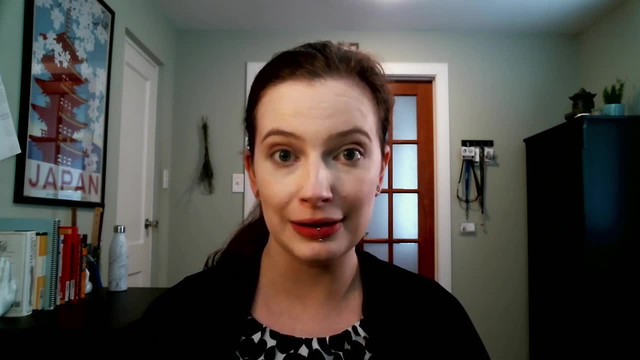 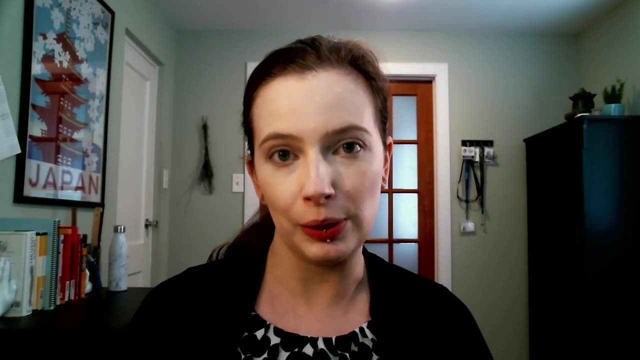 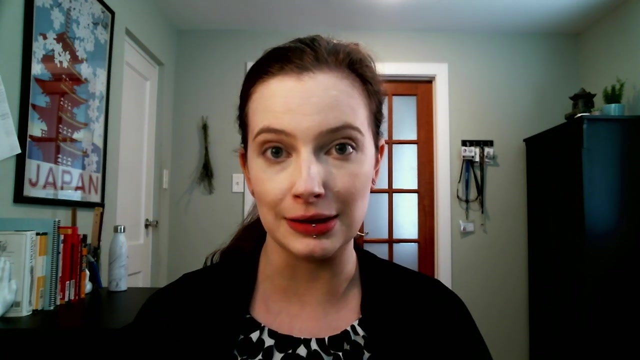 interpret in monotone. You should interpret tone of voice as well as emphasis. There's a difference between why do you need more pain medicine versus why do you need more pain medicine. Why do you need more pain medicine? That's an example of difference. 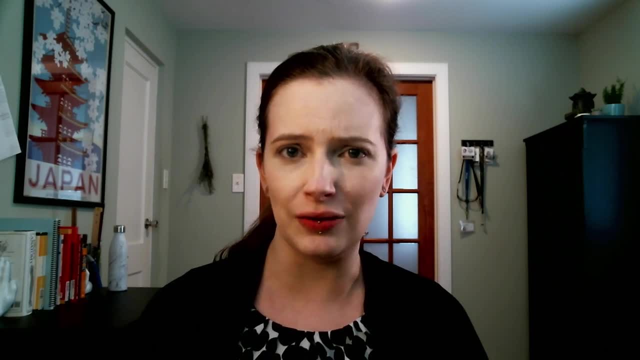 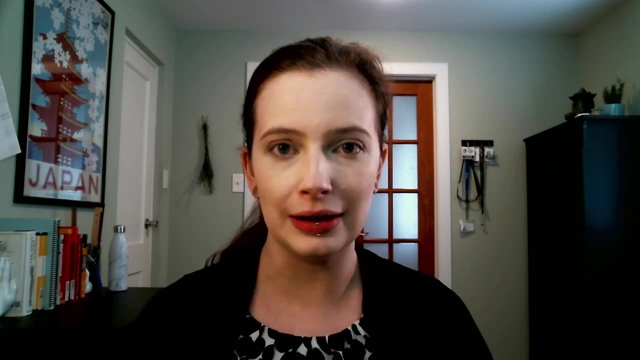 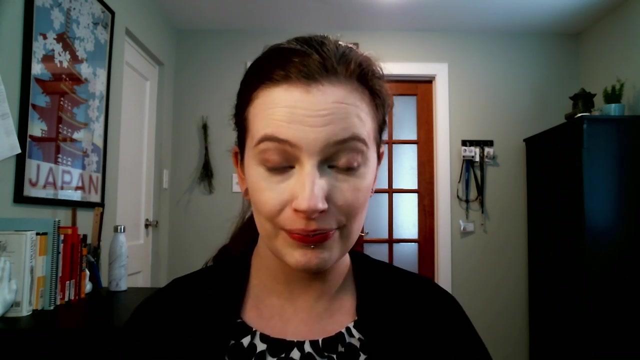 If someone's angry, they're going to go. I'm really angry. You need to interpret: I'm really angry, not I'm really angry. This actually brings me to my next point is: if you're practicing with a partner and someone is reading off the script as you practice, try and put some oomph into it. 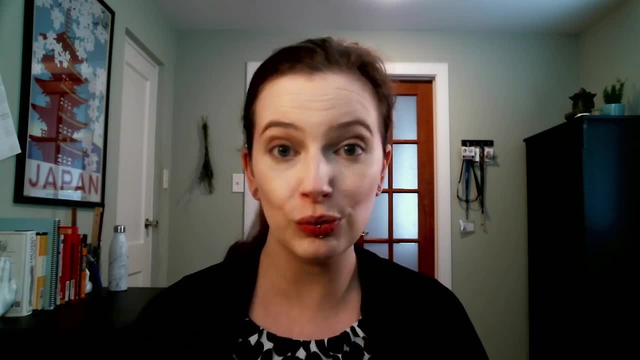 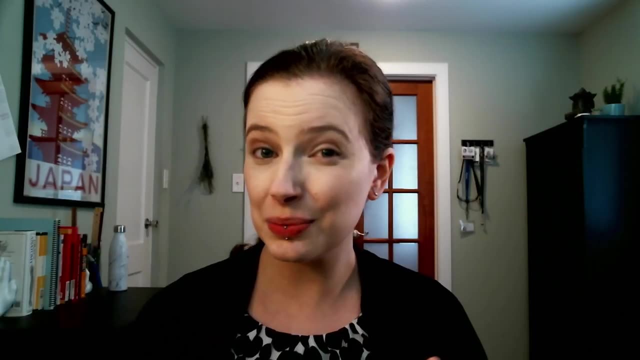 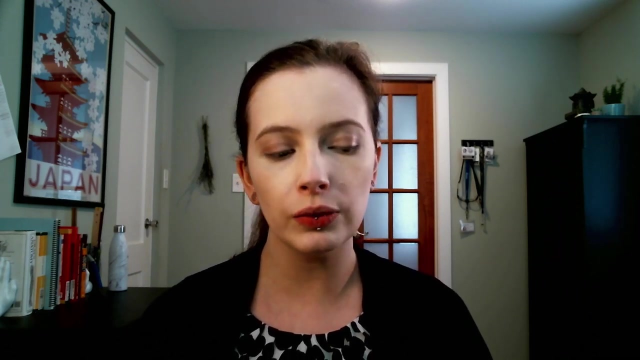 put some emotion into that. Be sure that when you're reading the script, you're putting yourself in that person's shoes And you're able to convey tone. If someone's angry in the interpreting script that you're reading, if someone's upset, you should convey those emotions. So not only is this going to 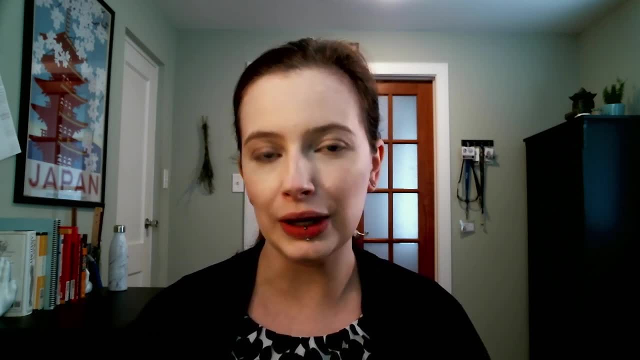 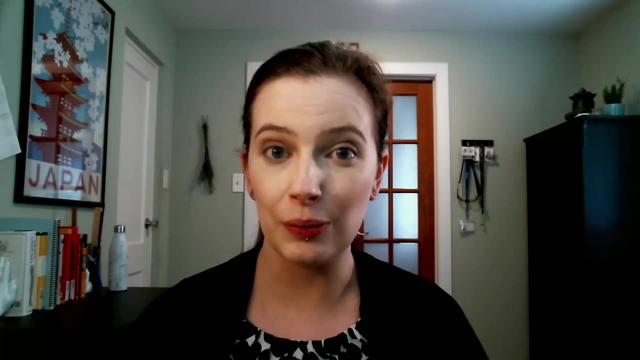 help you with one interpreting tone. it's also going to help you with putting yourself in other people's shoes, empathizing with other people. I really, really think that as interpreters, we undervalue emotional intelligence and all those different soft skills that we utilize. 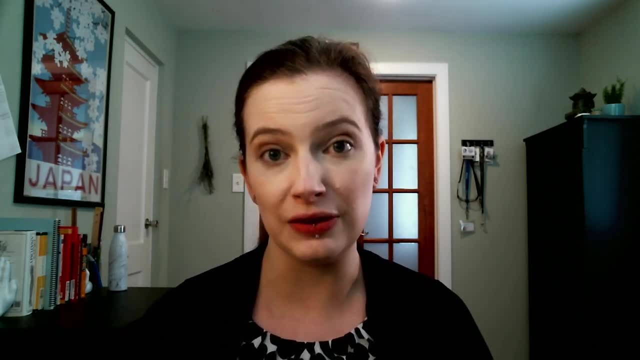 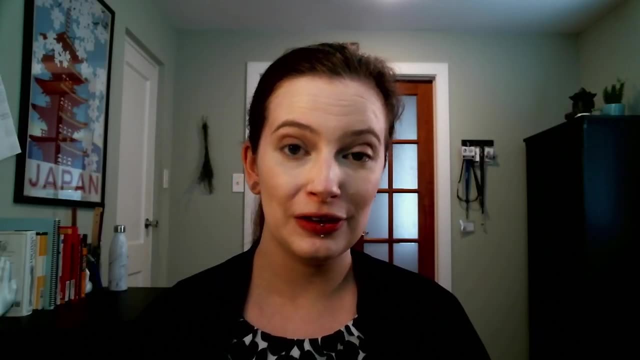 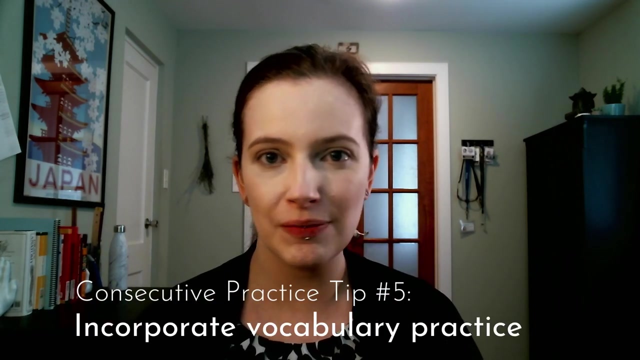 a lot in interpretation, So this is a great opportunity for you to practice with that and for you to be able to put yourself in someone else's shoes. And my last quick tip for practicing a consecutive interpretation- to make the most of your practice- is: incorporate some vocabulary. 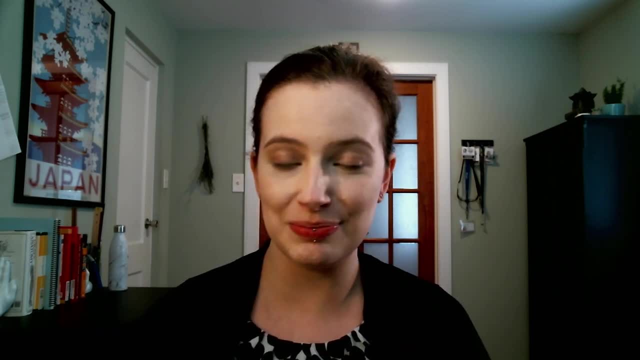 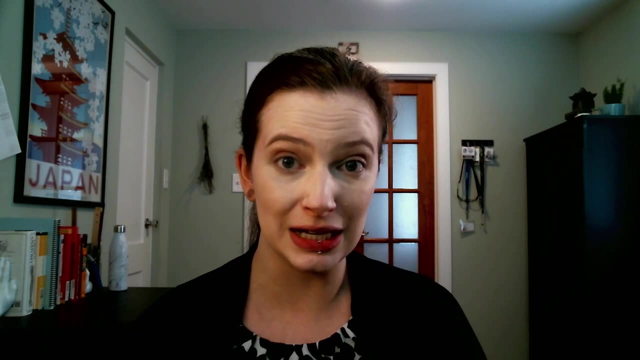 exercises. Now, this doesn't mean that you have to stop practicing with your script and do a vocabulary exercise. This means that one if you come across an unknown term, instead of ignoring it, you can stop practicing with your script and do a vocabulary exercise.